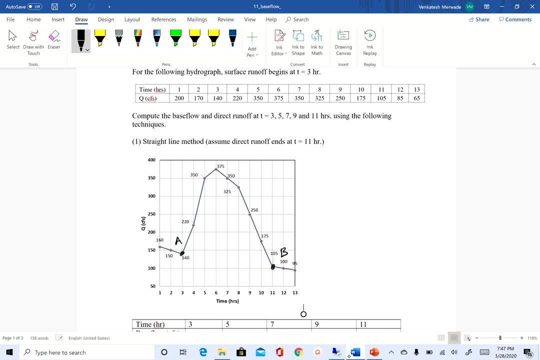 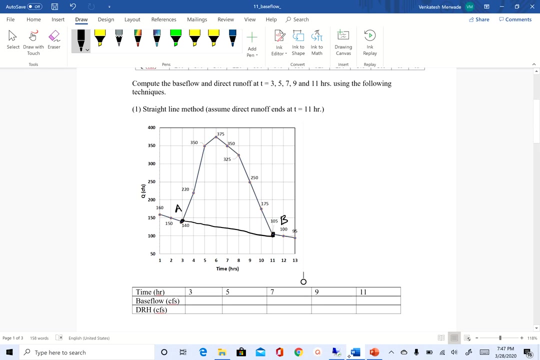 runoff starts and B is when it stops. so the straight line method says that you just join points A and B with a straight line. so you do that. then what I am asking you is to find out the base flow at different time steps. so what we are going to do is we are going to find the 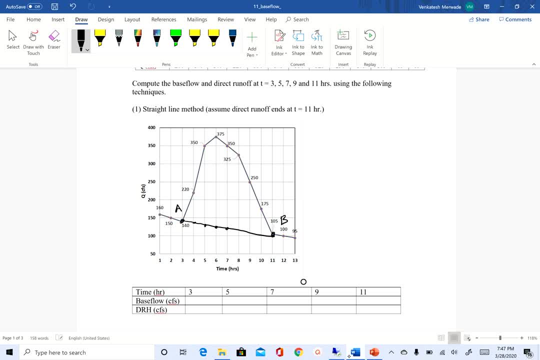 base flow at this times and in this table here I'm just asking you to report the base flow and the direct runoff at time equal to three hours, five hours, seven, nine and eleven. but i'll show you how to do it and I will only give you few. 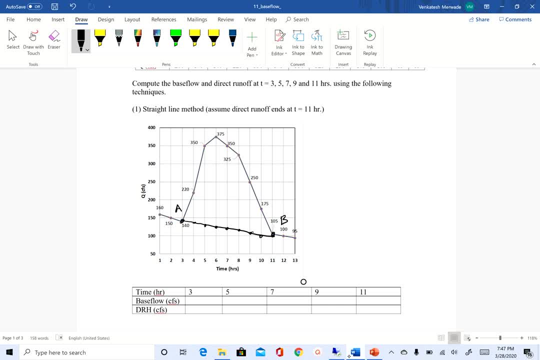 numbers, and then the rest you can do on your own. so we know that the value at A is 140, which is at time equal to 3, so this is going to be 140 and the hydrograph also has 140. so there is no direct runoff at this point. and, as I 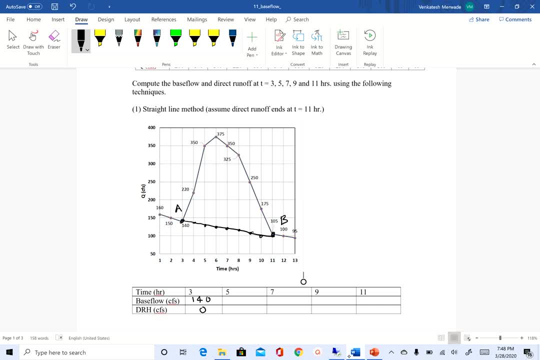 said, this is when the direct runoff starts. so the direct runoff starts on the of hydrograph value is 0, okay, and the base flow is 40, so let's see how we can get the values at 5, 7, 9 and 11. so to do that, what I'm going to do is I'm going 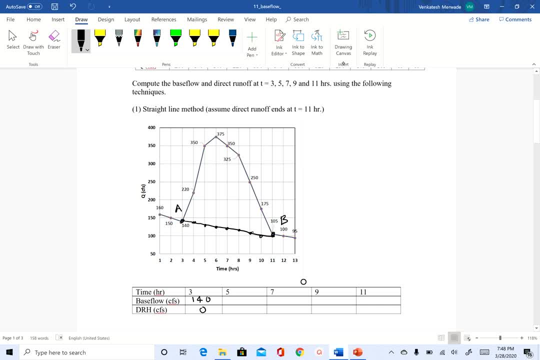 to find the slope of line a, b, so that slope will be 140 minus 105, that's the value of base flow at a and b. and then we have eight. so let's see 1, 2, 3, 4, 5, 6, 7, 8,, eight warm intervals. and if you do, that go to the boardū and this will show Here that here for the three-chapter program we will do two lessons, 1 th four, Morning in the afternoon, 6 in afternoon, Z, five in the afternoon and 6 in the afternoon, 7 in the afternoon, 8 hours in the afternoon and seven hours in the afternoon, and two lesson in the afternoon and 20 minutes in the afternoon. and the next week I'll be learning more and 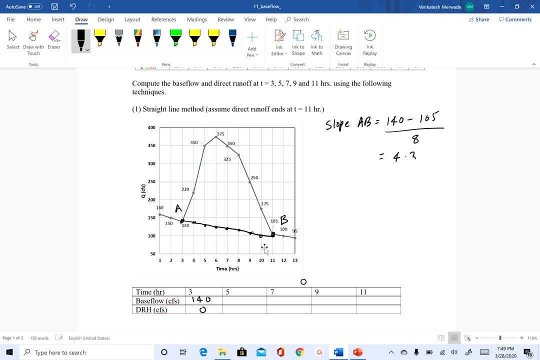 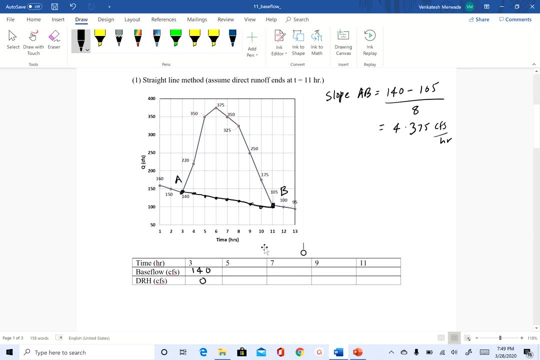 what you get is 4.375 CFS per hour. okay, so to get the value at 5 time equal to 5 hours, what you have to do is B at 5 is 140 minus 2 times that slope, so 2 times. so I'm using 2 because 140 is the value. 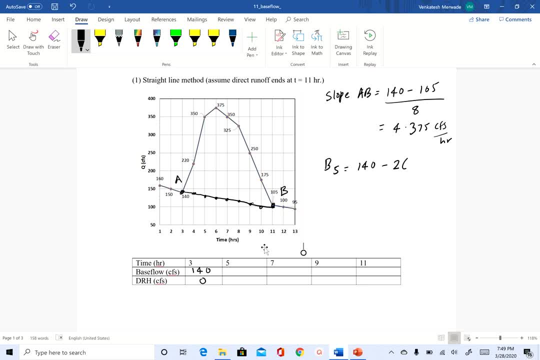 at t equal to 3 hours, and we are interested in t equal to 5 hours. so 2 times the slope at a B or slope of a B, so 4.375. and if you do that what you get is- I'm going to do this on my calculator here- 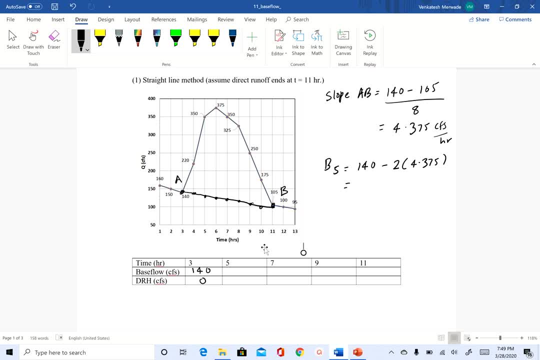 131.25. so this will be 131.25 and the direct runoff will then be, so this value will be at t equal to 5, the total flow is 350. so 350 minus 130, 1.25 will be the direct runoff value at t equal to. 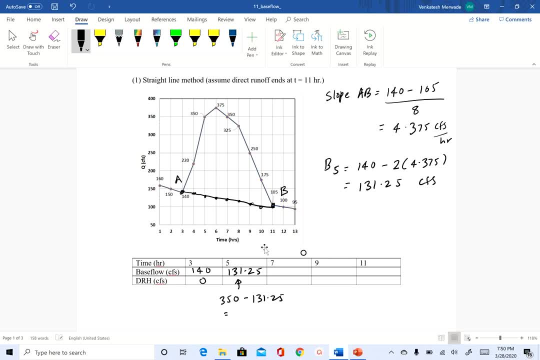 5 hours and that comes to that's two hundred and eighteen point seventy five CFS. so, similarly, for baseflow at seven, you will do one forty minus four times the slope for B, base flow at t, equal to nine hours, you will do, I'll do.